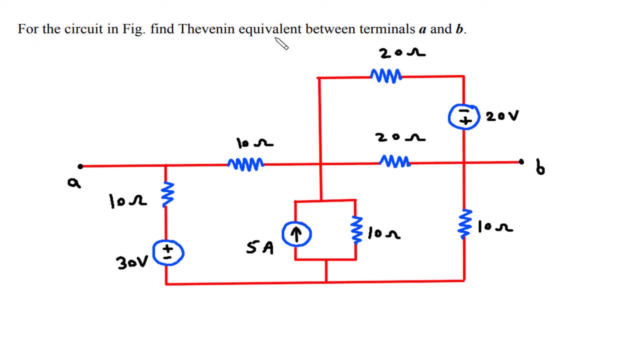 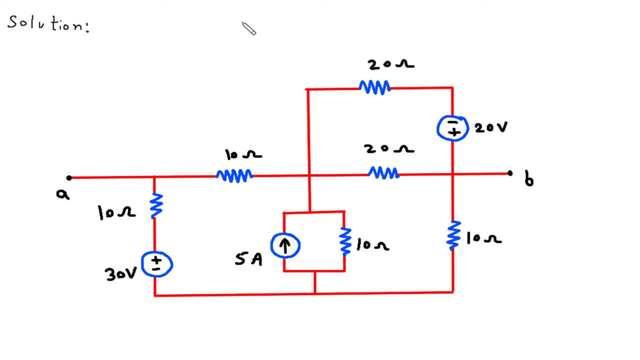 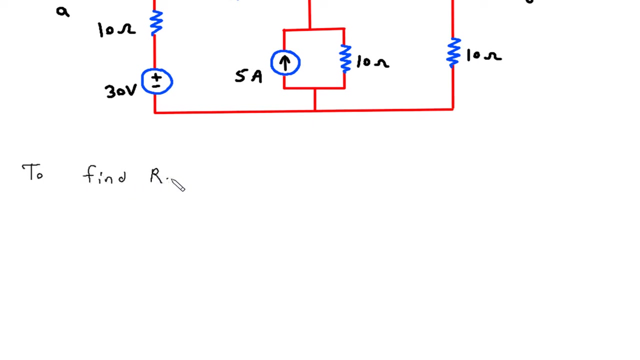 For the circuit in figure. find Thevenin equivalent between terminals A and B. Solution: First of all we will redraw the circuit. Now we have to find Rth and Vth. So to find Rth we will turn off all the sources. 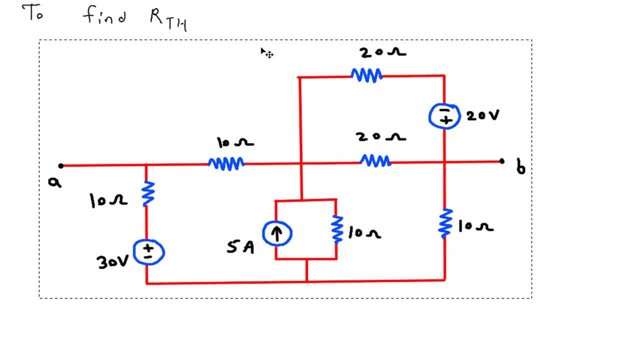 Vth will be short circuited. Cth will be open circuited. This is current Sre, so it will be open circuited. This is voltage Sre, so it will be short circulated Now, as we can see that. 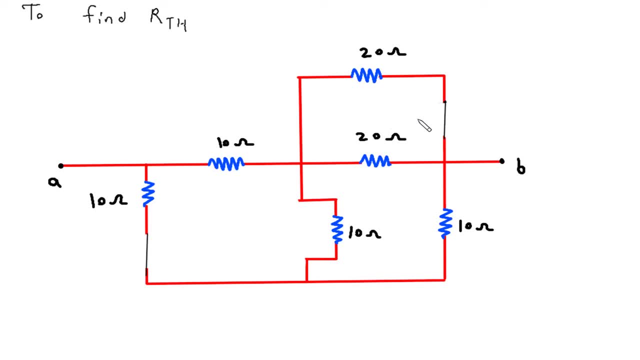 This 20 ohm is in parallel with this 20 ohm, So it will be short circuited. So this will be 10 ohm. this will be 10 ohm now. this will be 10 ohm now, this 10 ohm, and. 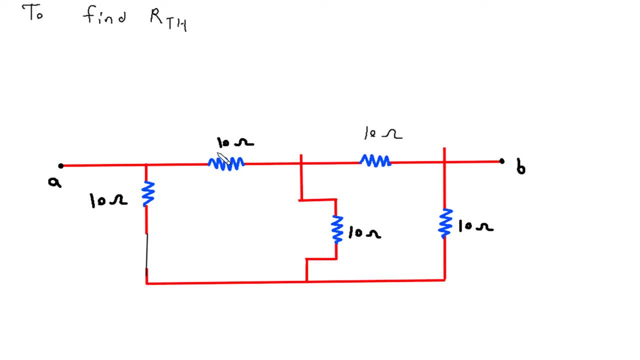 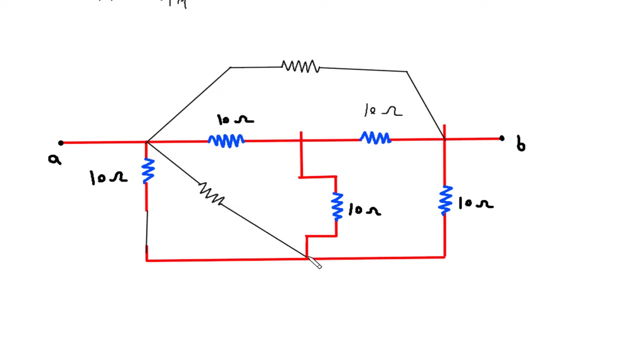 this: 10 ohm. this forms a star connection. this 10 ohm: 10 ohm, 10 ohm. this forms a star connection. we will convert it into its equivalent Delta connection. So it's equivalent Delta will be like this: 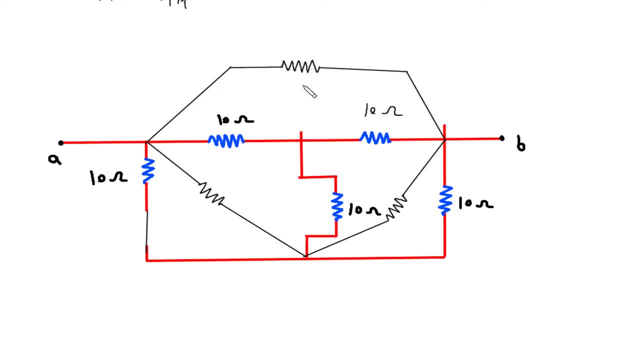 Now let's say this is 10 ohm, This is Ra or directly. we will calculate here. so this will be 10 into 10.. So 10 into 10, 10 into 10 plus 10 into 10, 10 into 10 plus 10 into 10, 10 into 10 divided. 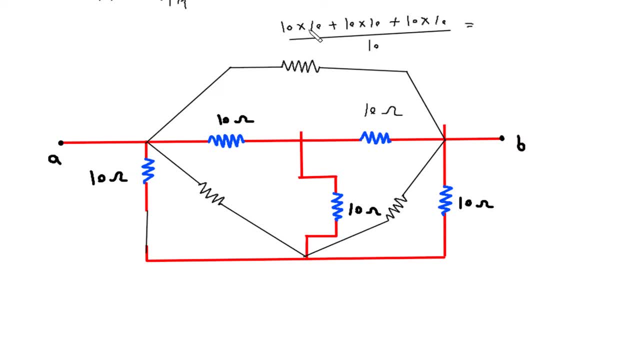 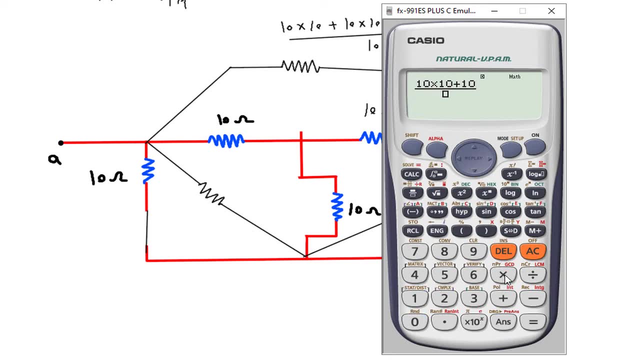 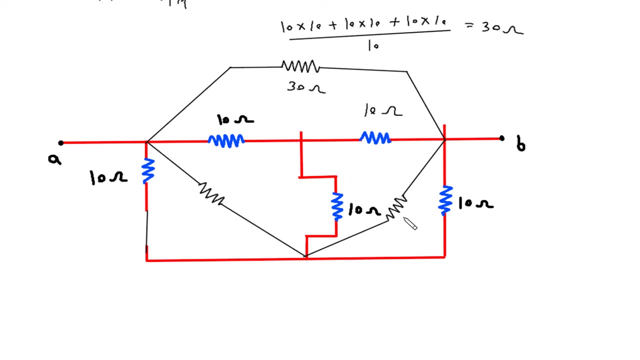 by 10.. So this will be 10.. 10 into 10 plus 10 into 10 plus 10 into 10 divided by 10. This will be 30 ohm, So this will be 30 ohm. Also, this will be 30 ohm and this also 30 ohm. 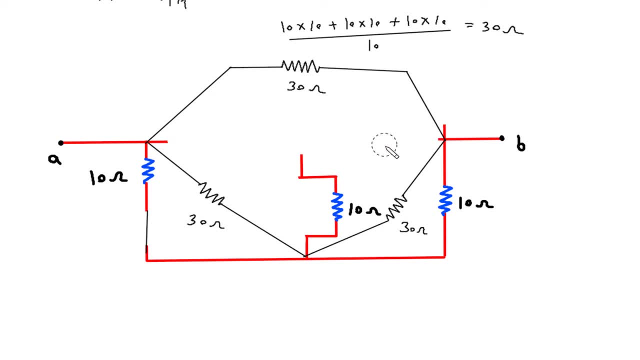 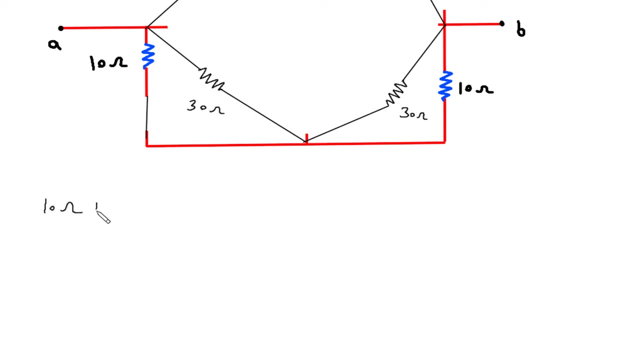 Now we will erase this Now as we can see that this 10 ohm is in parallel with this 30 ohm. So 10 ohm parallel with 30 ohm will be 10 ohm parallel with 30 ohm. 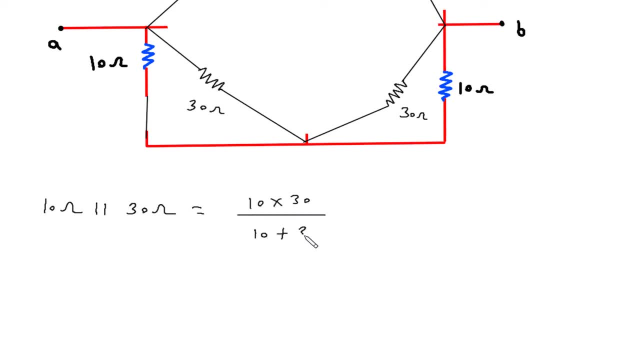 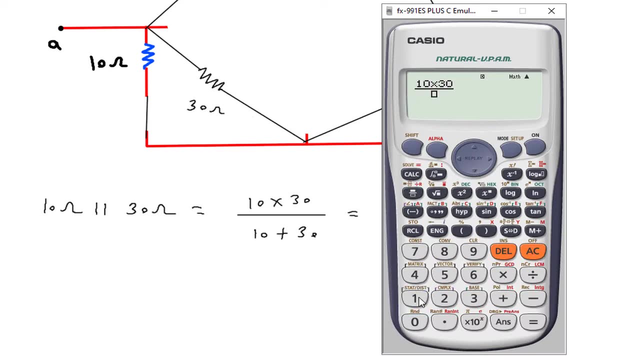 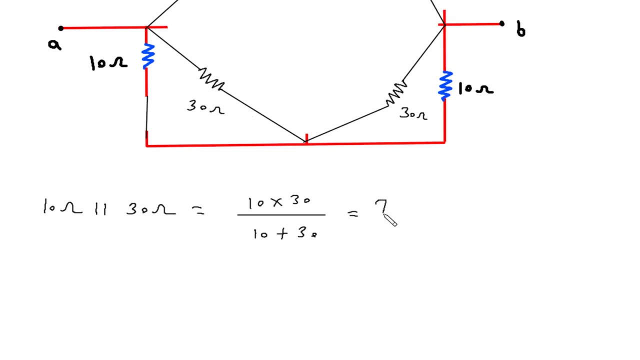 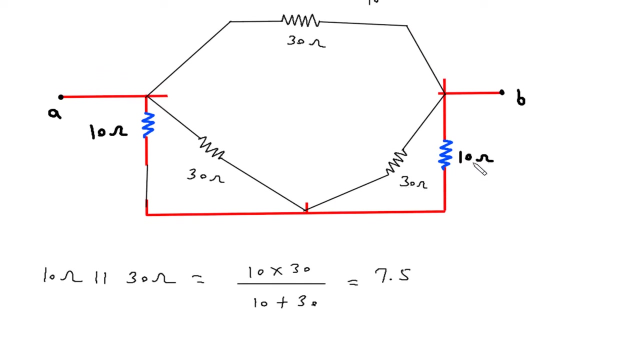 So 10 into 30, divided by 10 plus 30.. 10 into 30.. 10 plus 30.. 15 by 2 or 7.5, directly 7.5, and this will be. this is also 30, parallel with 10 ohm. 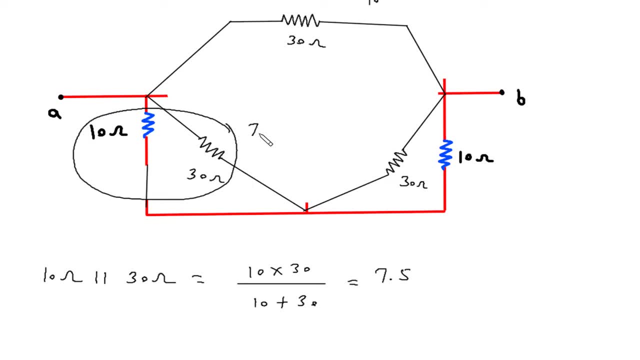 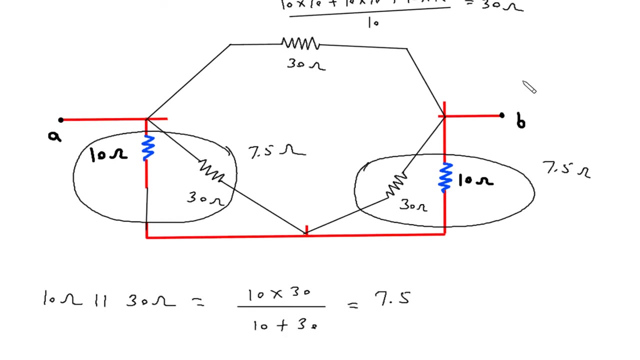 So this will be 7.5.. So this will be 7.5 ohm and this is also 7.5 ohm and these are in series. So this total will be 15 ohm. So this will be 15 ohm parallel with 30 ohm. 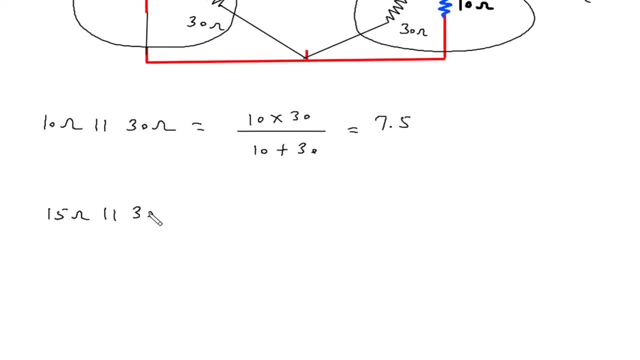 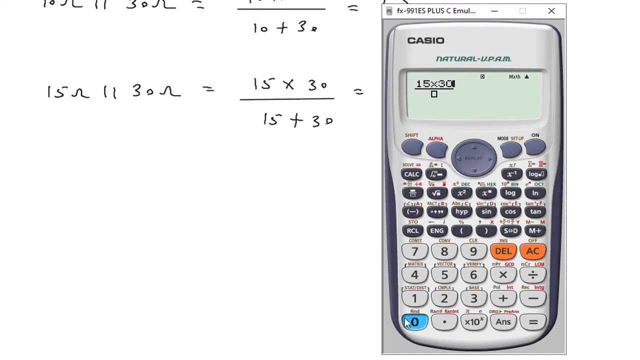 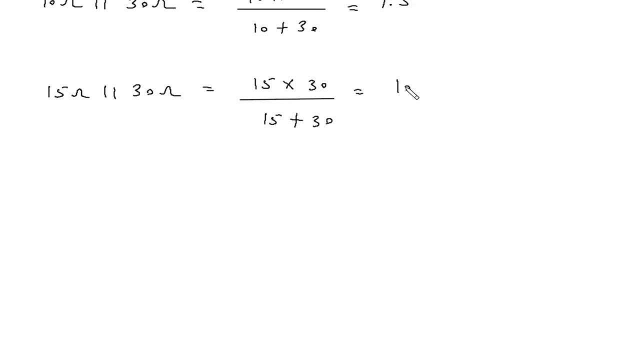 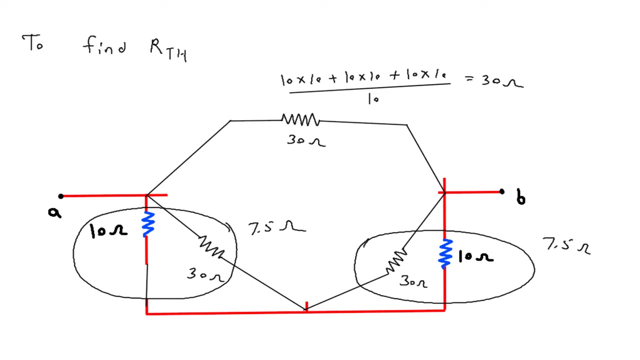 15 ohm parallel with 30 ohm. this will be 15 into 30 divided by 15 plus 30.. 15 into 30 divided by 15 plus 30. So it is 10 ohm. Therefore, There is a difference between A and B, which is Rth. 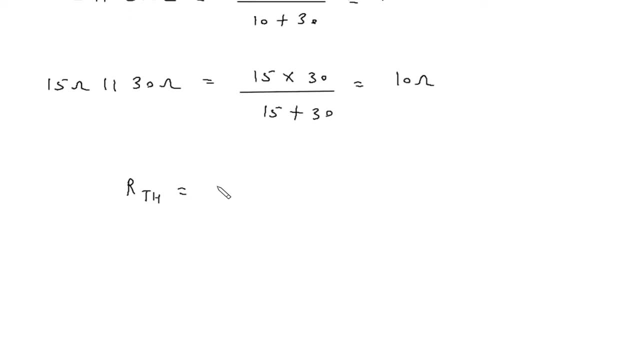 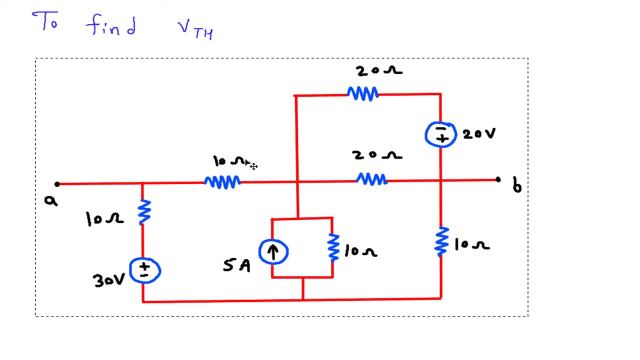 So Rth is equal to. Rth is equal to 10 ohm. Next, we have to find Vth. So to find Vth, To find Vth, we will. we will consider this circuit and now we will convert this current source into its equivalent voltage source. 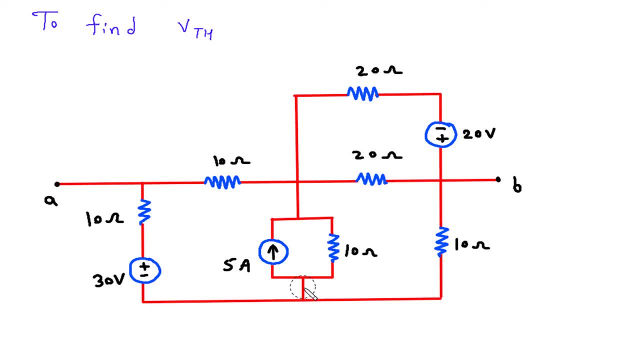 So here this will be a voltage source. This will be a voltage source in series with this resistor. This will be positive and this will be negative. V is equal to I into R, So 5 into 10 is 15.5.. 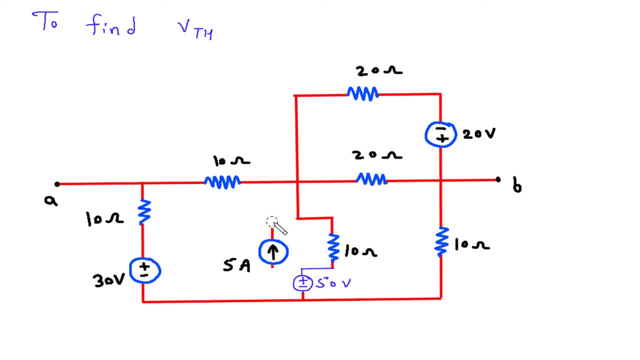 This will be 50 volt. This will be 50 volt. Now we will convert this voltage source into its equivalent current source. So here currently it is in series with this 20 ohm. So the current source will be in parallel with this 20 ohm. 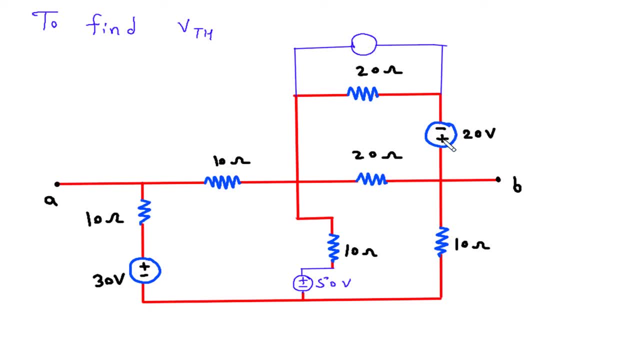 So current source will be in this direction: positive and negative. So The direction of current source will be like this: And current is equal to V by R, Where V is 20 and R is 20.. So this will be 1 ampere. 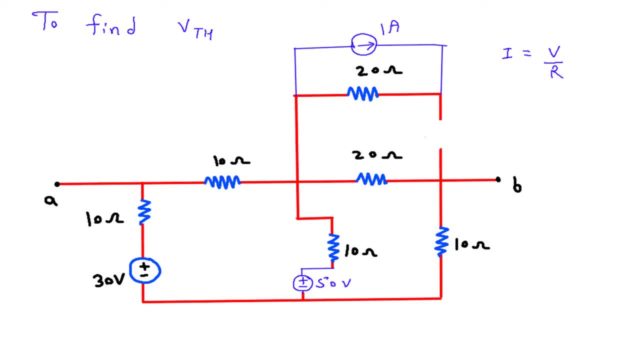 And this will be turn off. Now this 20 ohm parallel with 20 ohm, So this will be 10 ohm, This will be 10 ohm. Now again we can convert this 1 ampere into its equivalent voltage source. 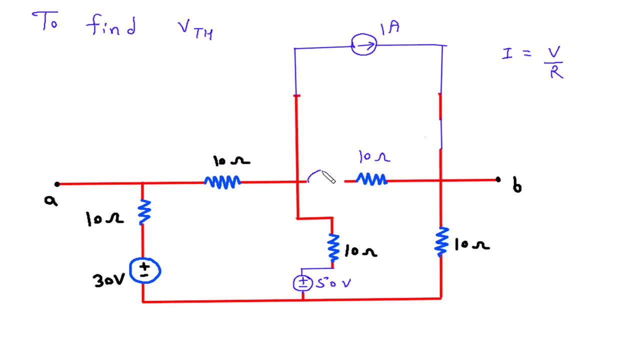 So here this will be a voltage source In series with this 10 ohm. This will be positive and this will be negative. V is equal to I into R, So 1 into 10 is 10 volt. This will be positive and this will be negative. 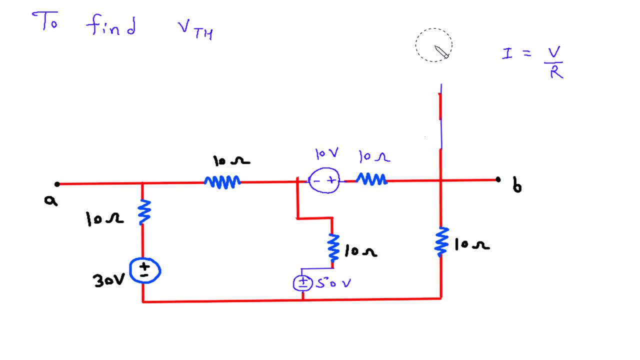 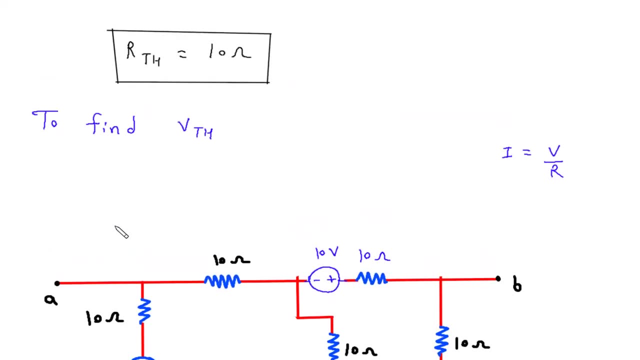 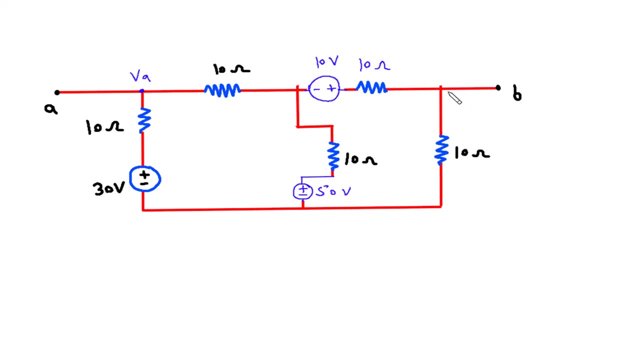 V is equal to I into R, So 1 into 10 is 10 volt. Now here we can apply mesh analysis. The voltage between A and B will be Vth. So let's assume this is node VA and this is node VB. 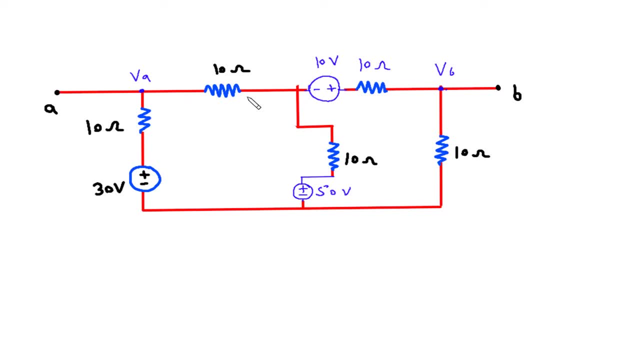 We can apply mesh analysis or nodal analysis here. So let's assume this is ground Vb, We will apply nodal analysis. Let's say: this is current I1.. This is current I2.. This is current I3.. This is current I4. 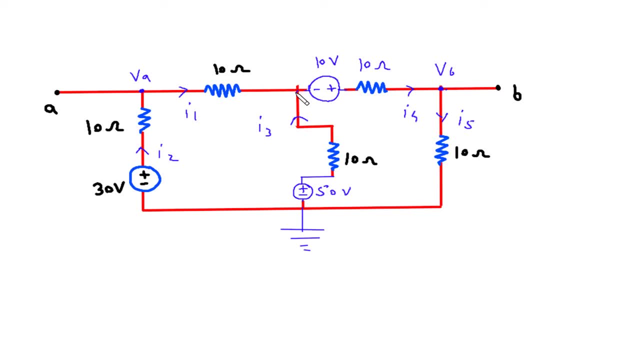 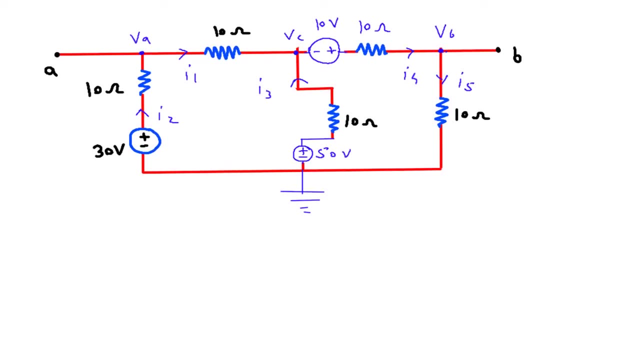 And this is current I5.. Let's say this is node VC. Now we will apply: apply KCL at node VA. Apply KCL at node VA. So summation of all the entering current at this node is I2.. I2 is equal to I1.. 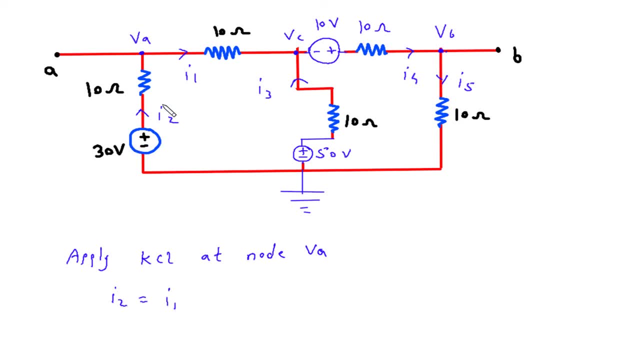 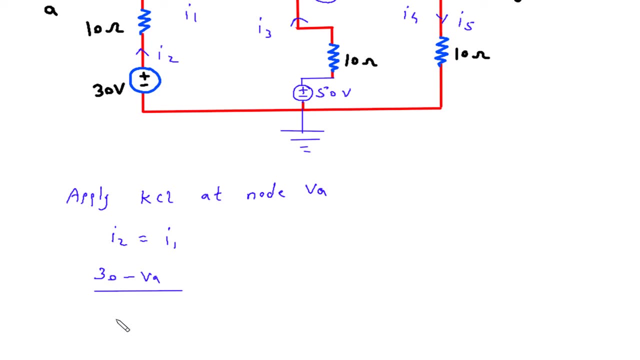 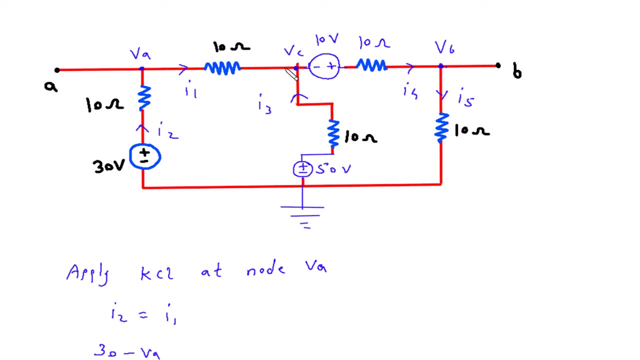 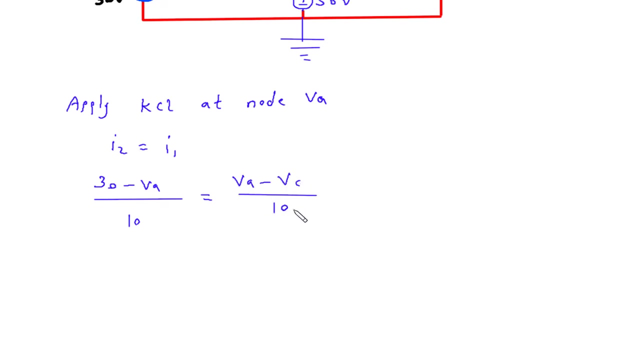 I2 is equal to I1.. I2 is 30 minus VA. 30 minus VA, divided by 10 ohm Is equal to I1.. I1 is VA minus VC. VA minus VC by 10.. VA minus VC by 10.. 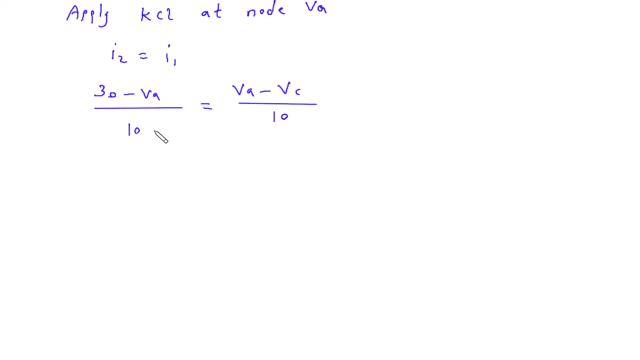 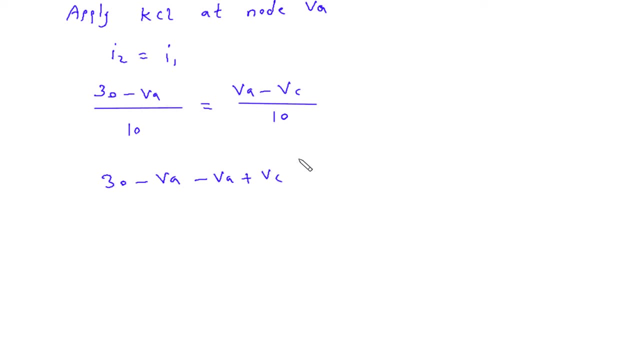 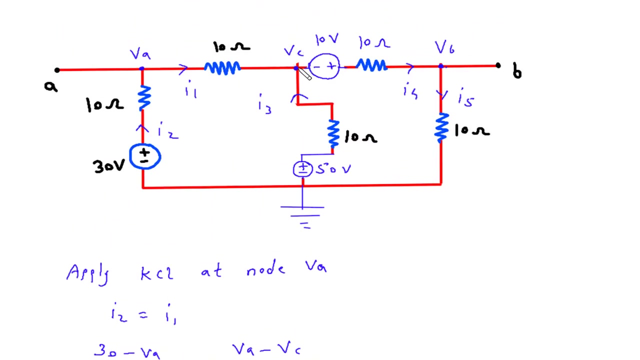 30 minus VA minus VA plus VC is equal to 0.. So this will be minus 2 minus 2. VA plus VC is equal to minus 30.. Let's say this is equation number 1.. Now we will apply KCL at node VC. 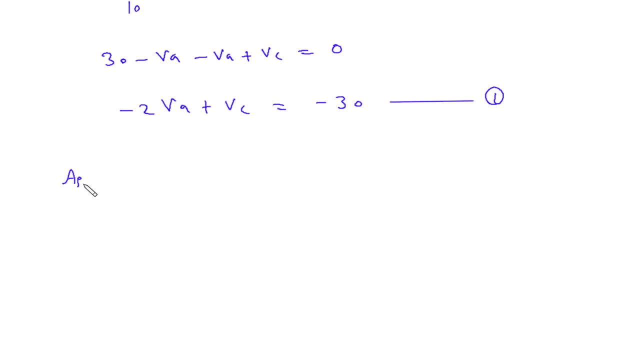 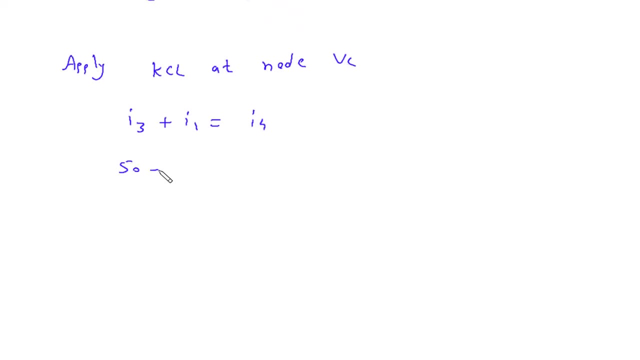 by 10 plus I1.. I1 is VA minus VC by 10.. VA minus VC by 10 is equal to I4.. I4 is VC minus VB by 10.. This will be VC. VC will be 10 to the power 5.. 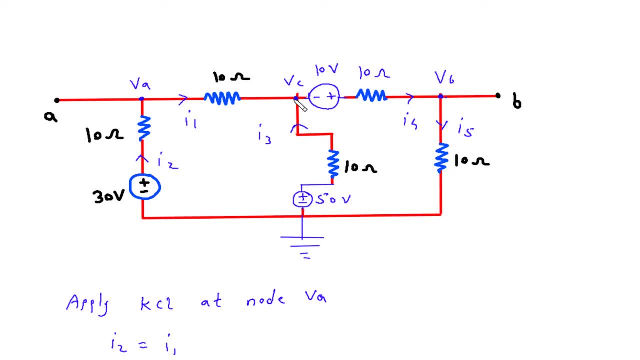 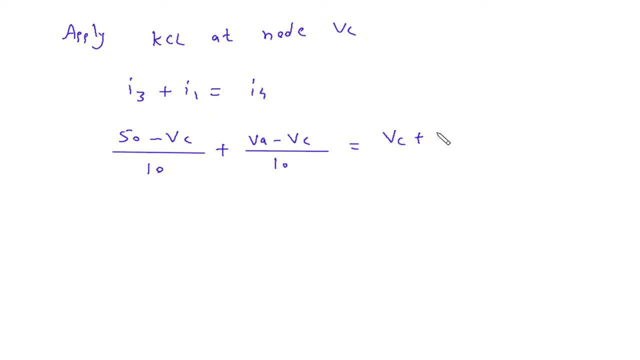 VC is also equal to I1.. VC is also equal to I2.. So VC is equal to I4.. So VC is VB by 10.. So VC is equal to I4.. be Vc minus, this will be Vc plus 10, Vc plus 10 minus Vb. Vc plus 10 minus Vc plus 10 minus. 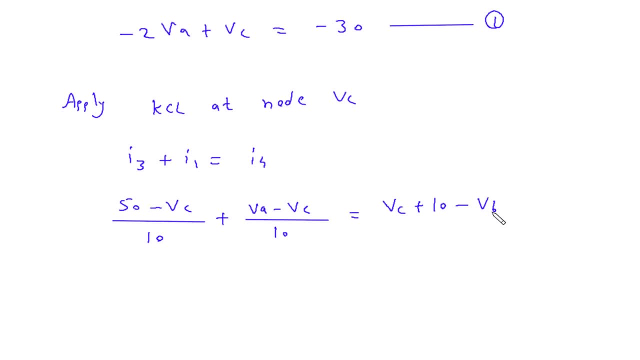 Vb minus Vb by 10 ohm, Now this will be 50 by 10, so this will be 5 minus Vc by 10 plus Va by 10. minus Vc by 10 is equal to: or directly. we can simplify this by cancelling this 10. 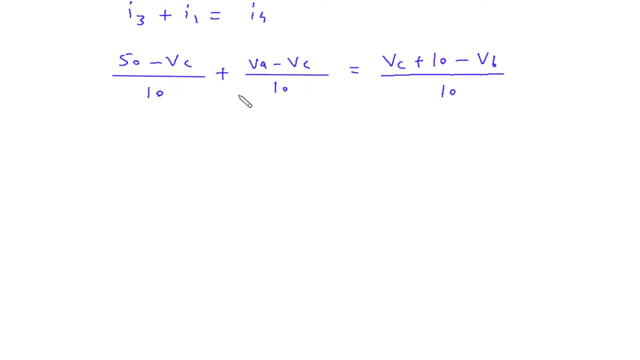 by 10, this 10 will get cancelled with this 10, this whole 10 will be cancelled with this 10, so this will be 50 minus Vc, then plus Va, 50 minus Vc, plus Va, minus Vc, minus Vc. 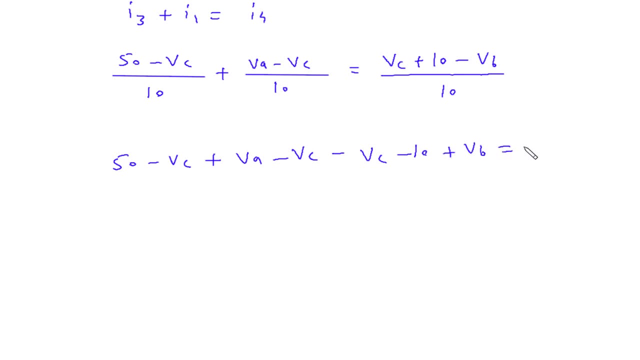 minus 10 plus Vb is equal to 0.. Now this will be Va plus Vb, and this will be Vb minus Vc, and this will be minus 1 minus 1, minus 2, minus 2 minus 3, so minus 3, Vc is equal to this. 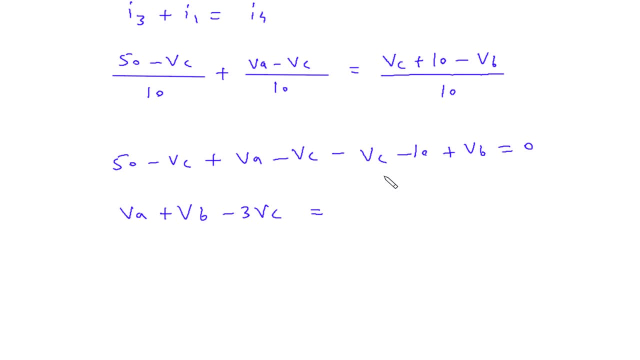 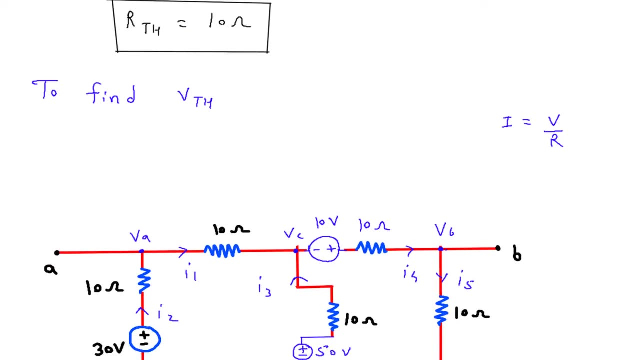 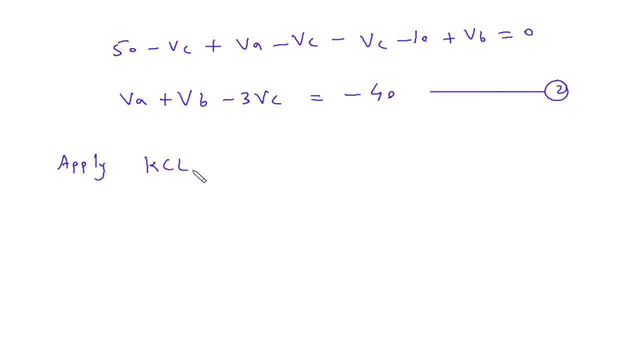 will be 50,. 50 minus 10 will be 40, so minus 40. Let's say this is equation number 2.. Now we will apply KCL at node Vb. Apply KCL at node Vb. Apply KCL at node Vb. 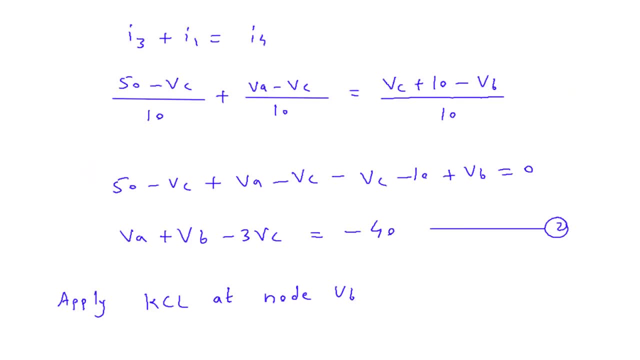 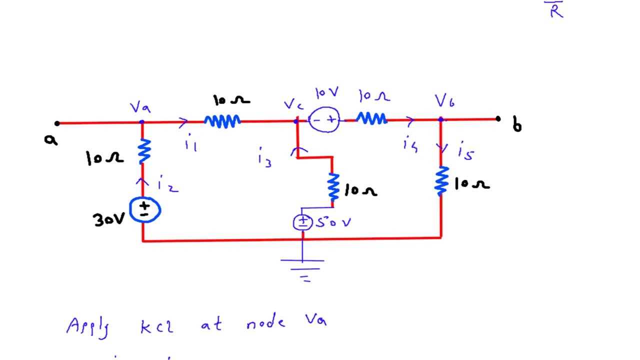 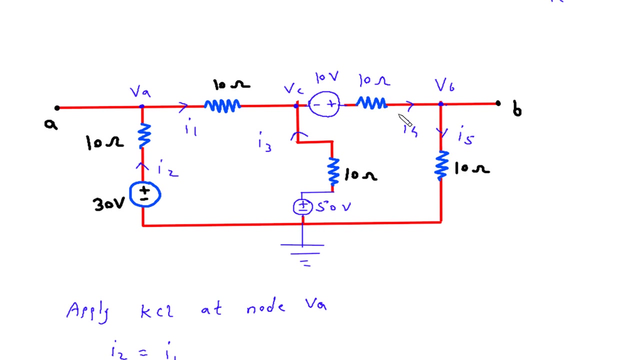 So entering current at this node is I4 and leaving current is I5. So I4 is equal to I5.. I4 is equal to I5, now I4 is I4 is Vc, Vc plus 10 minus Vb. 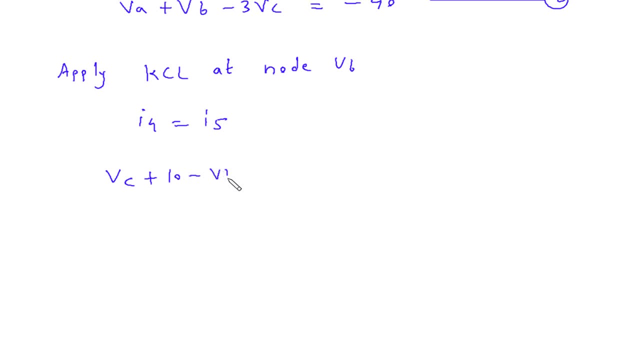 Vc plus 10 minus Vb. 10 minus VB divided by 10 ohm is equal to I5.. Now this I5 is VB minus 0 by 10.. VB minus 0 by 10.. Now this 10 and this 10 will get cancelled. 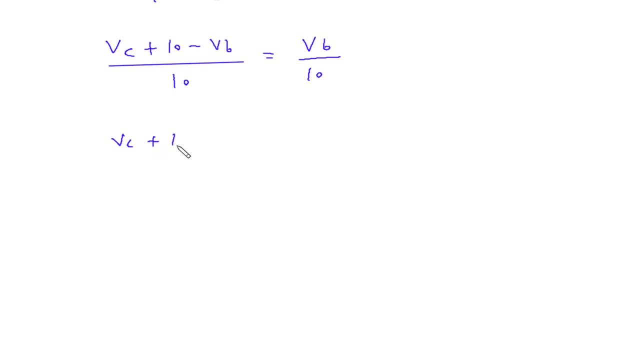 So this will be: Vc plus 10. minus VB is equal to, or directly minus VB is equal to 0.. So this will be: minus 2 VB plus Vc is equal to minus 10.. Let's say this is equation number 3.. 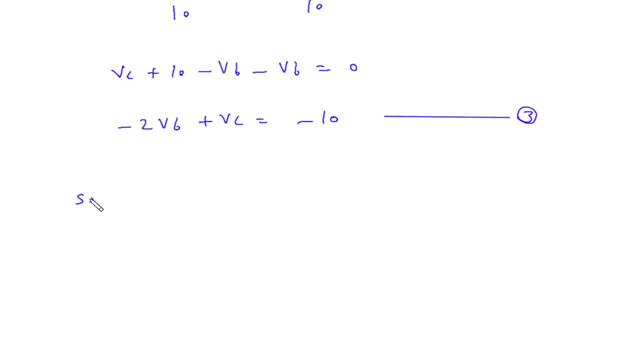 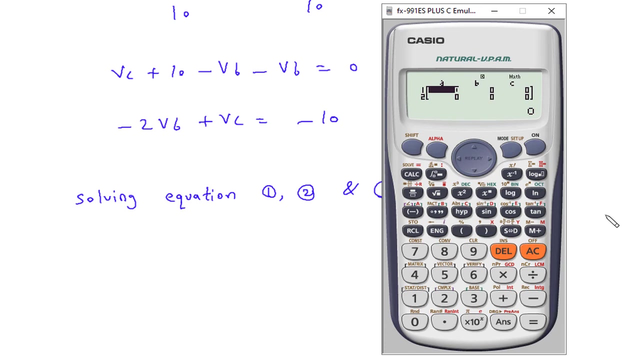 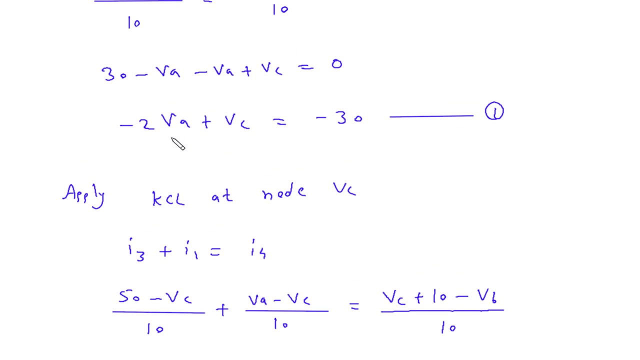 Now we will solve equation 1,, 2 and 3.. Solving equation 1, 2 and 3, we get mode 5 1, mode 5 2, because there are three unknowns. So from equation number 1 this will be minus 2. 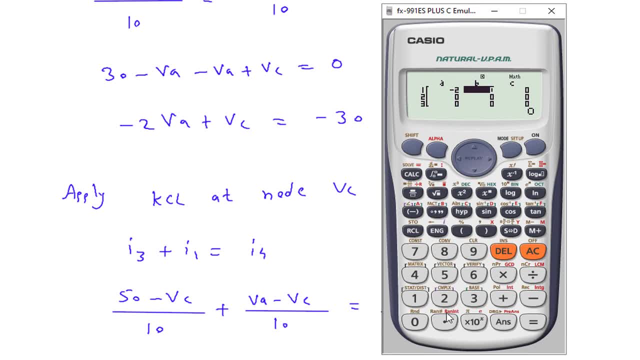 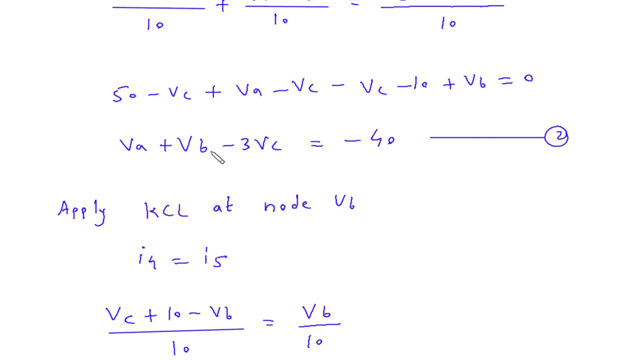 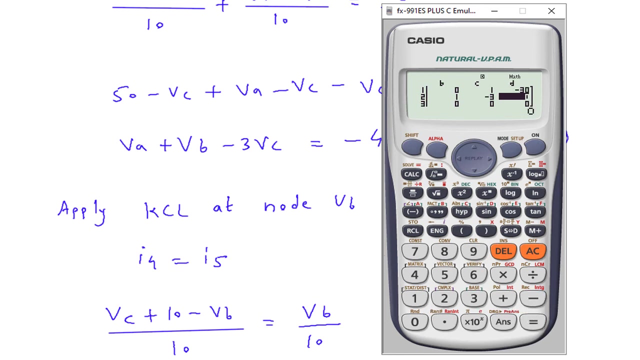 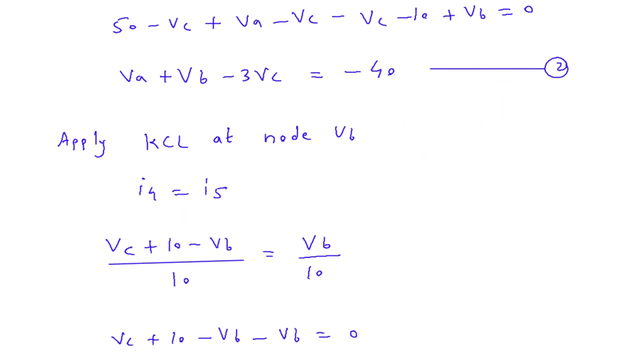 minus 2, then VB is absent. so 0, then 1 minus 30, then from equation number 2, this will be 1, 1 minus 3, 1 1 minus 3 minus 40 minus 40, then from equation number 3, this will be: